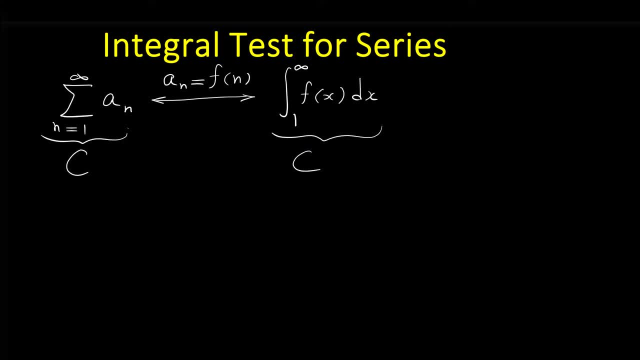 then the series is also convergent, And if the integral diverges, then the series diverges. So actually the series and the integral have the same behavior. If one of them converges, the other one converges, Or if one of them diverges, the other one diverges. 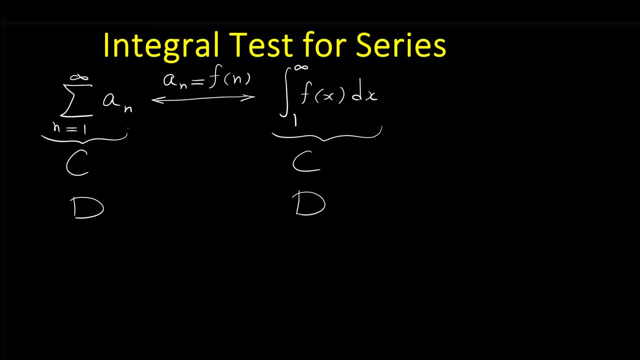 But note that you can use this test only if the function f of x, the function associated to the series, is continuous on the interval 1 to infinity positive. And finally, the function should be decreasing on the interval 1 to infinity. 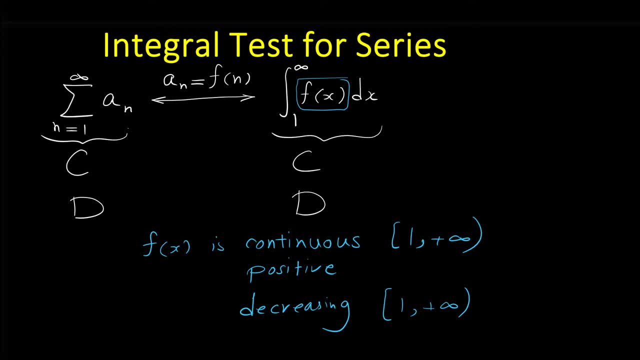 So if you want to use the integral test, first you have to use the integral test. You have to make sure that the function associated to the series is continuous, positive and decreasing. Then you can use this test to determine the convergence or divergence of series. 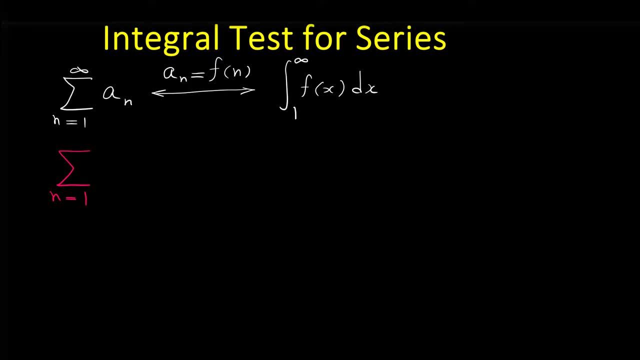 Let's do some examples with the integral test. Consider this series, sigma n, from 1 to infinity, of 1 over n squared. We want to use this test to determine the convergence or divergence of series. We want to use the integral test to determine the convergence or divergence of series. 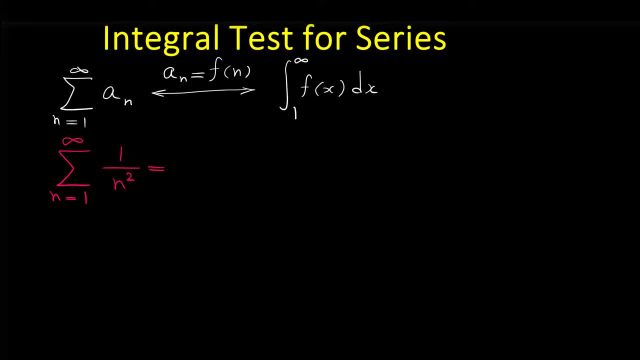 If we write a few terms of these series, the first term, if we plug in 1 for n, 1 over 1 squared, is 1.. The second term is 1 over 2 squared, which is 1 over 4.. 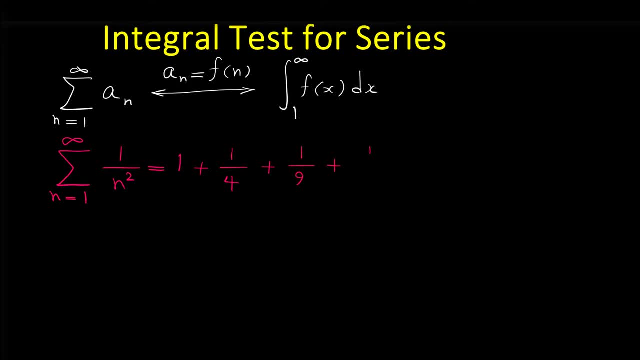 The third term is 1 over 9.. The fourth term is 1 over 16. And so on. As you can see here the terms of these series are positive and decreasing, So we can use the integral test for these series. 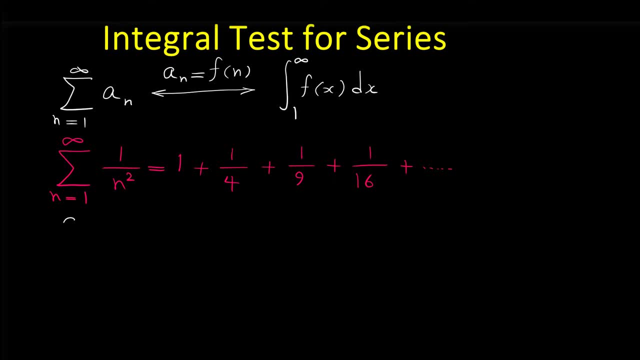 The relevant integral to these series is integral from 1 to infinity, of 1 over x to the 2 dx. For finding this integral, we can bring x to the 2 to the numerator and write it in the form of x to the negative, 2 dx from 1 to infinity. 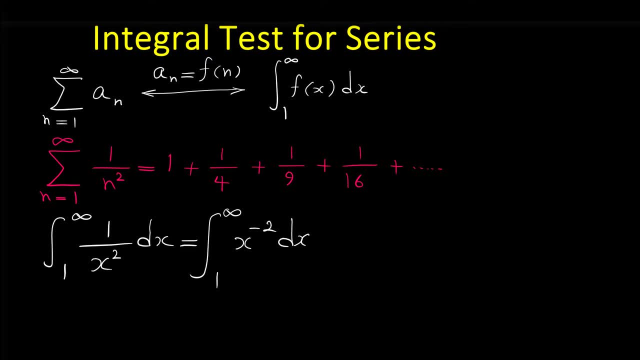 Integral of x to the negative 2 dx, based on the power of four integrals, is x to the power of negative 2 plus 1 over negative 2 plus 1.. Negative 2 plus 1 is negative 1. And the derivative is negative 1.. 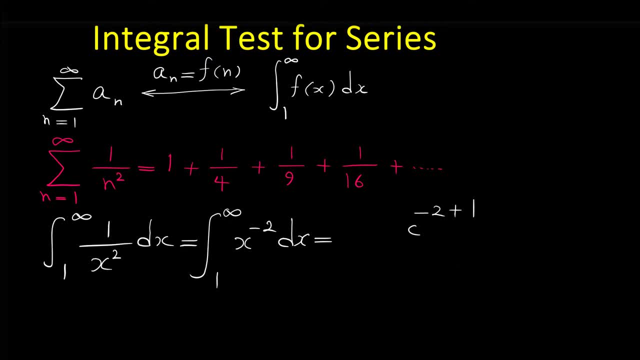 And the denominator is also negative 1.. So the integral equals to x, to the power of negative 1 over negative 1.. But because this integral is improper integral, we have to write this in the form of limit. b approaches infinity from 1 to b. 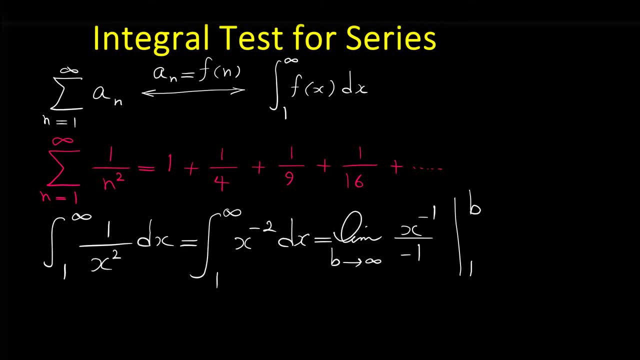 Now, if we plug in b for x, this equals to limit of b to infinity. Now, if we plug in b for x, this equals to limit of b to infinity. Now, if we plug in b for x, this equals to limit of b to infinity. 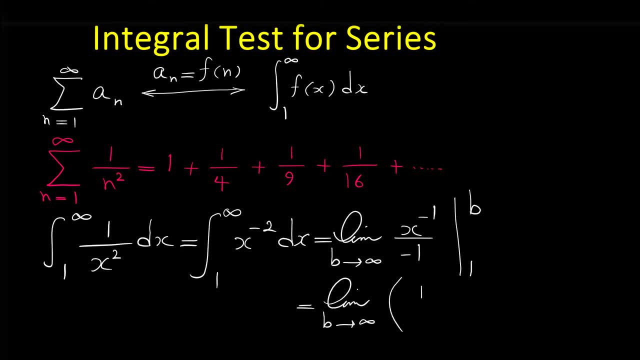 b approaches infinity of b to the negative, 1 over negative, 1 minus. If we plug in 1 for x, 1 to any power is 1 over negative, 1 is negative 1.. Note that b to the negative 1 is 1 over b. 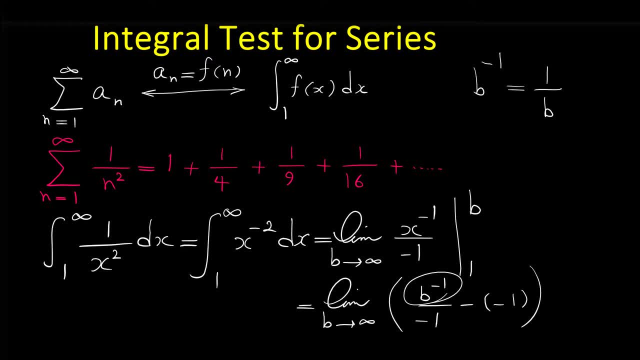 And because b approaches infinity, in this limit 1 over infinity approaches 0.. And so the limit of b to the negative 1 over negative 1 is 0.. 0 minus negative 1 equals 1.. Because the integral is convergent, from the integral test we can conclude that the given series is also convergent. 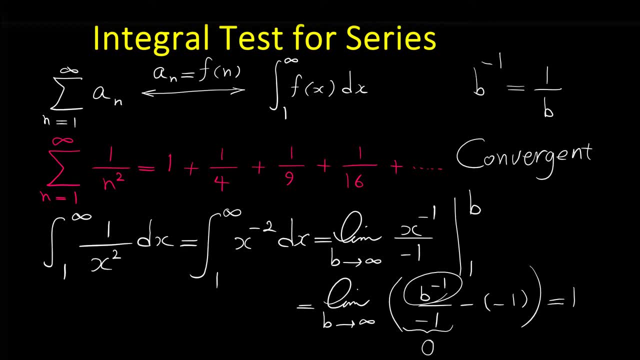 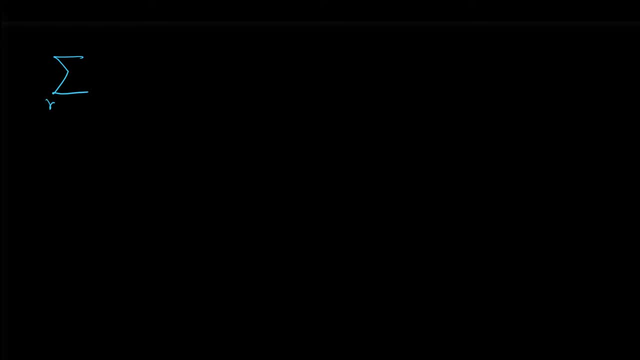 Thank you for watching. let's try another example: sigma n from 1 to infinity, of 1 over n. probably you know these series and you know this is harmonic series, which is divergent. but here we want to use the integral test to prove that the harmonic series is divergent. if we write the first, 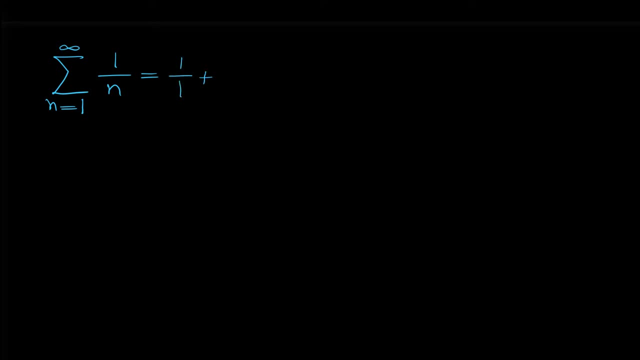 few terms of these series. the first term is 1 over 1, the second term is 1 over 2, the third term is 1 over 3, and so on. as you can see here, all the terms of these series are positive and they are. 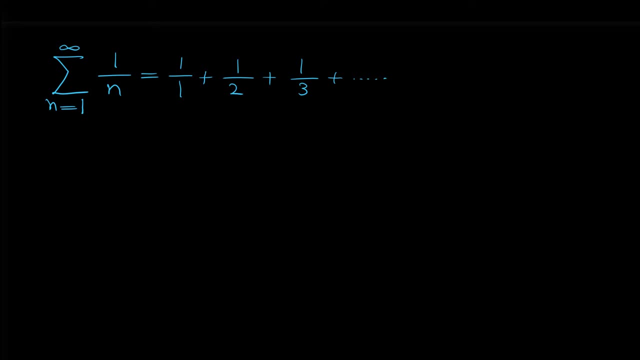 decreasing, so we can use the integral test for these series. the integral associated to this series is integral from 1 to infinity, infinity of 1 over x dx. we know that integral of 1 over x dx is ln of x and because this is an improper integral, we have to set it up in this form of limit b. 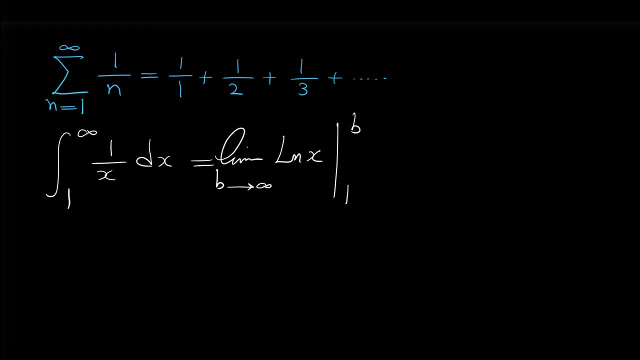 goes to infinity from 1 to b. now if we plug in b for x, we have limit of ln of b minus ln of 1. b approaches infinity. limit of ln of b when b goes to infinity is infinity. remember the graph of ln of x. If you look at the graph of ln of x, you can see that If you go far to the 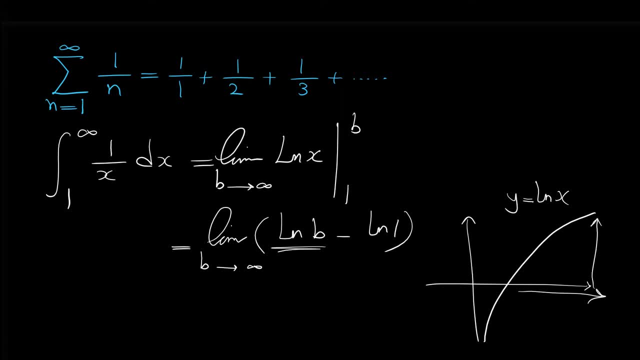 right. the y values of ln of x gets larger and larger. They increase without bond, And so ln of b, when b goes to infinity, is infinity, So this limit equals infinity. Note that ln of 1 is 0.. And because ln of b, when b goes to infinity, is infinity, this limit is infinity. 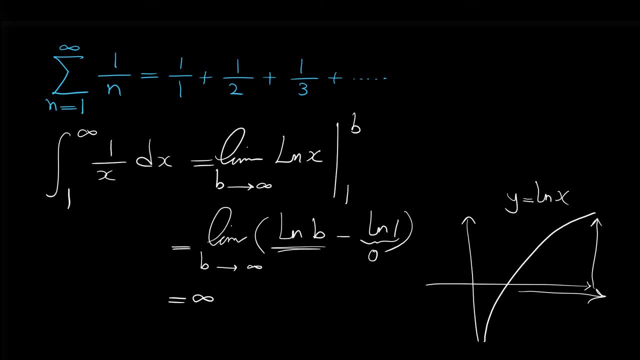 And because the integral diverges, we can conclude about the harmonic series that the harmonic series is our limit. When the integral is convergent, the series is convergent. When the integral is divergent, the series is also divergent. Consider this series, sigma n, from 2 to infinity, 1 over. 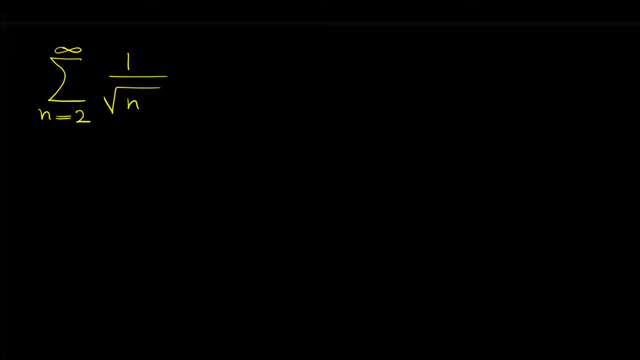 square root of n. Note that in this series n starts from 2.. But still, we can use the integral test for this series And it doesn't change anything. The only change that we should do in the integral test is that we have to also start our integral. 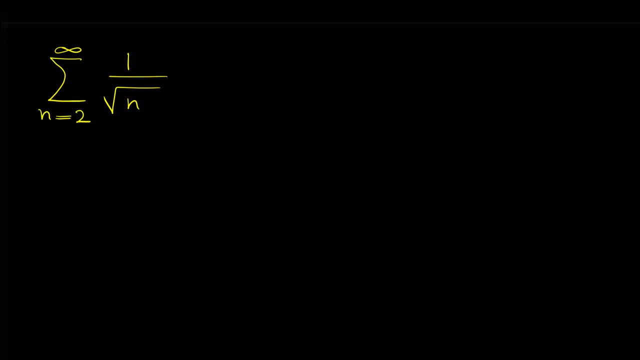 from 2.. If we write the first few terms of this series, the first term is 1 over square root of 2.. The second term is 1 over square root of 2.. The third term is 1 over square root of 3.. 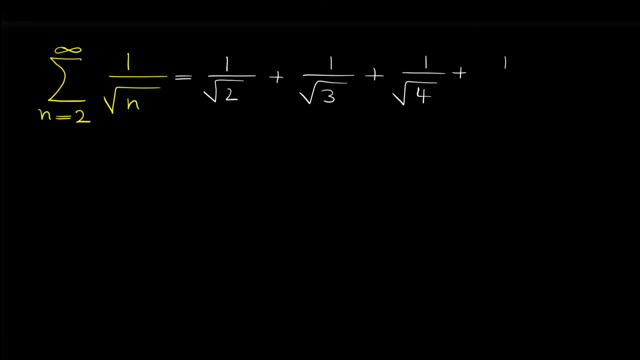 The fourth term is 1 over square root of 4,, which is 1 over 2.. The fourth term is 1 over square root of 5, and so on. Again, as you can see, all the terms of this series are positive and they are decreasing. 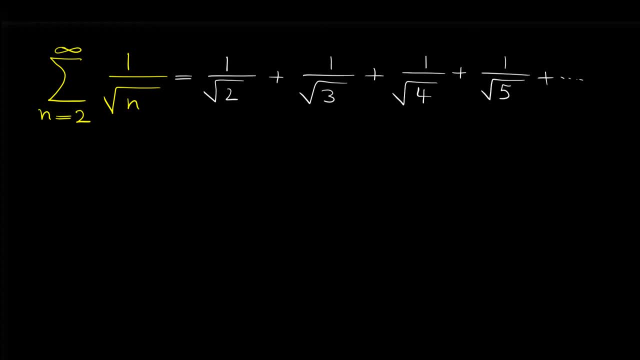 So we can use the integral test for this series. The relevant integral to this series is integral from 2 to infinity to infinity. instead of starting the integral from 1 here we start from 2, because the series also is started from 2, integral from 2 to infinity and the 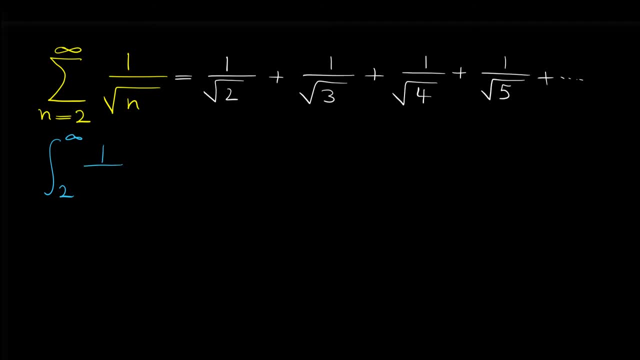 function associated to this series is 1 over the square root of X, DX. for finding this integral, first I rewrite the integral, the expressions in front of the integral, in the form of X to the power of negative 1 over 2. note that radical X is x to the 1 over 2, but because we bring the radical X from the denominator. 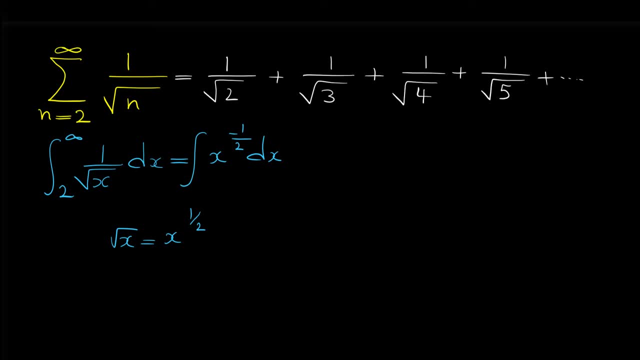 to the numerator, we have to make the power negative integral of X to the negative. 1 over 2 DX is integral of X to the negative. 1 over 2 DX is X to the negative. 1 over 2 DX is US period of omega, but the integral is: 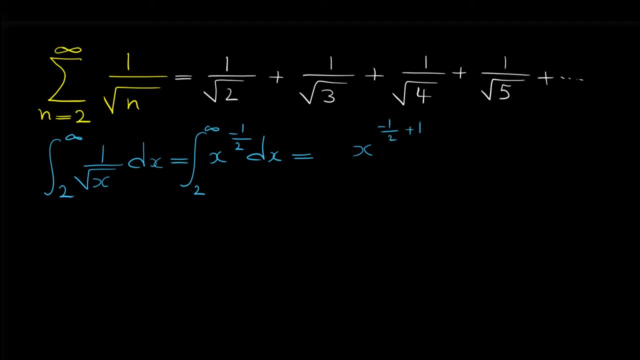 1 over x is x squared and the integral useful and as well as negative 1 power. all the other values are that the integral needed to равно is equal to, you know, x to the negative, 1 over 2 plus 1 over negative, 1 over 2 plus 1. negative 1 over 2 plus 1 is 1 over 2. 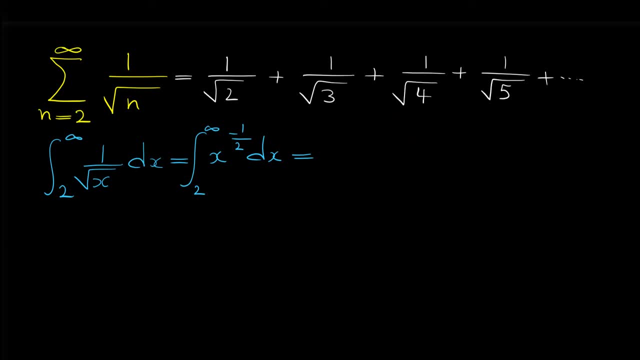 so this integral equals to x to the 1 over 2, all over 1 over 2, from 2 to b, which b goes to infinity. and we can simplify this and write this in the form of limit of 2: x to the 1 over 2. 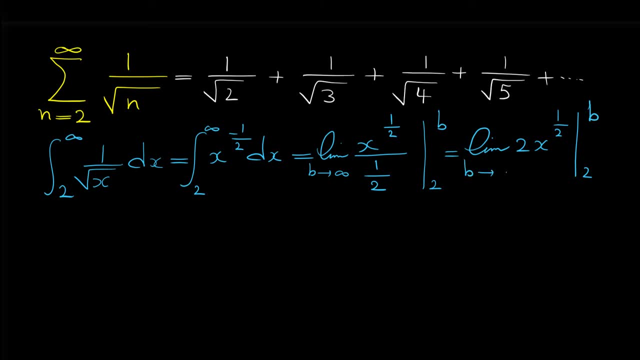 from 2, b and b approaches infinity, which this equals to limit of, if we plug in the upper one, b, 2 times b to the 1 over 2, minus 2 times 2 to the power of 1 over 2, because b approaches infinity, infinity, p is infinity to the power of 1 over 2. 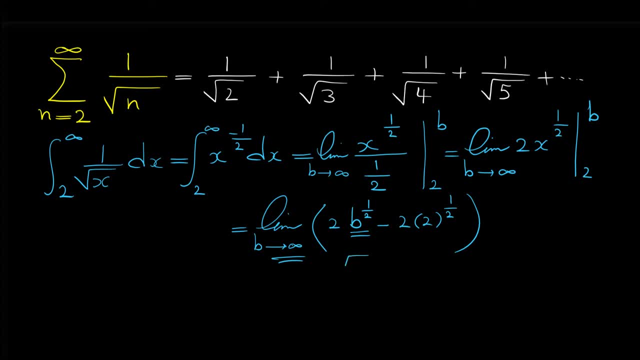 is infinity, because b to the 1 over 2 is actually square root of b and the square root of infinity is infinity. this limit equals infinity. because this limit does not exist, so the integral is divergent. and because the integral is divergent, so this series is divergent. 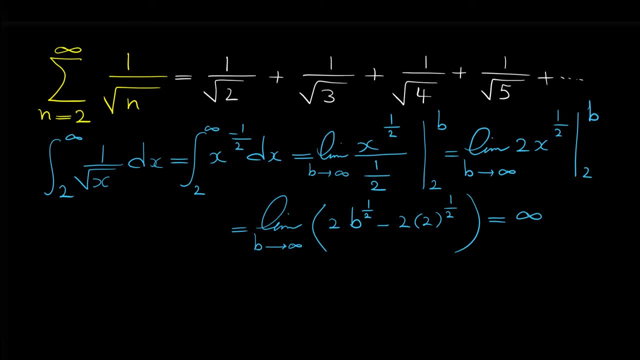 with the integral test. in general, we can prove that the series in the form of sigma 1 over n to the power of p. n starts from 1, 2 or any other number to infinity is convergent if the power p is greater than 1. 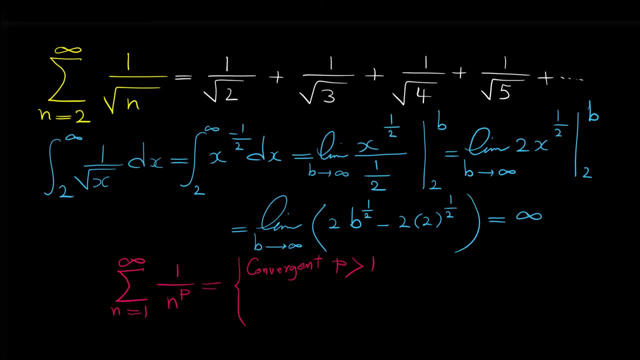 so convergence happens if the power of n is greater than 1.. so convergence happens if the power of n is greater than 1.. if the power p is greater than 1.. if the power p is equal to 1 or less than 1, then these type of series are divergent. 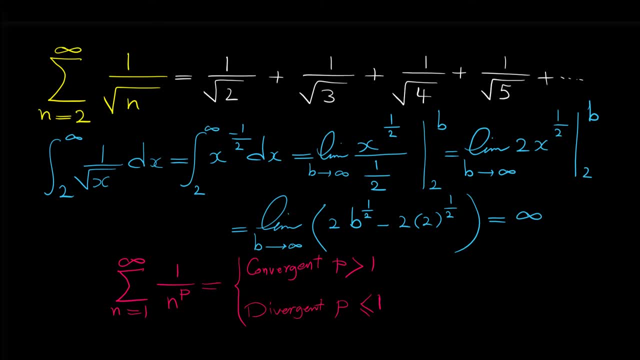 if the power n is less than 1.. we name these type of series p series, and it's a good idea to memorize this rule about the p series. if the power p is greater than 1.. if the power p is equal to 1.. 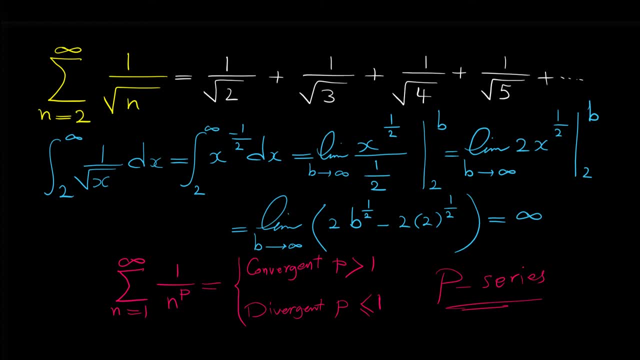 p series are convergent for the power n if the power n is greater than 1.. if the power p is greater than 1.. greater than one and are divergent for the powers less than or equal one. for example, series sigma 1 over square root of n. n from 2 to infinity. the power of n. 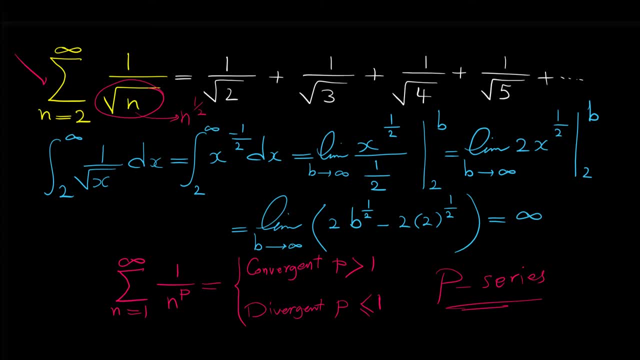 is one half, because the square root of n is actually n- to the power of 1 over 2, and because the power is less than 1, 1 over 2 is less than 1, based on the p series, based on the rule for p. 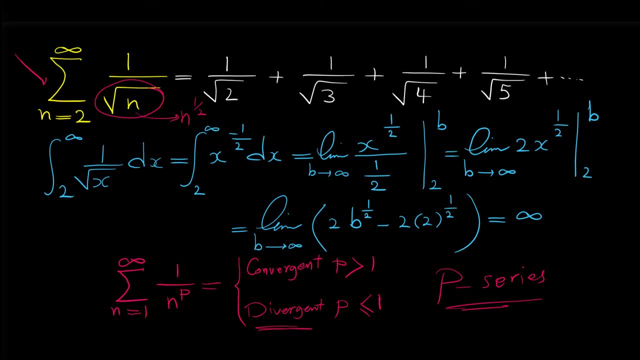 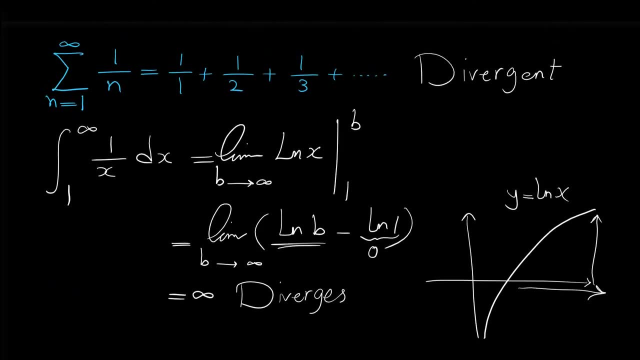 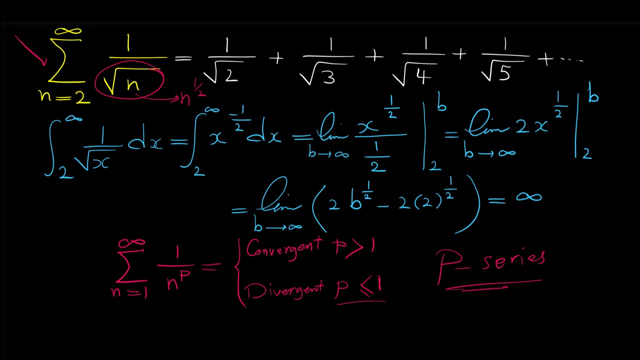 series, the series is divergent. if we look at the other examples that we did in this video, for example, if we look at the harmonic series that here we have the power of n here is 1 and based on the p series, when the power is 1, the p series is divergent. 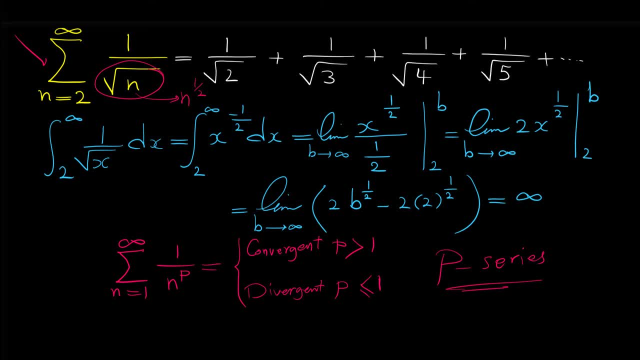 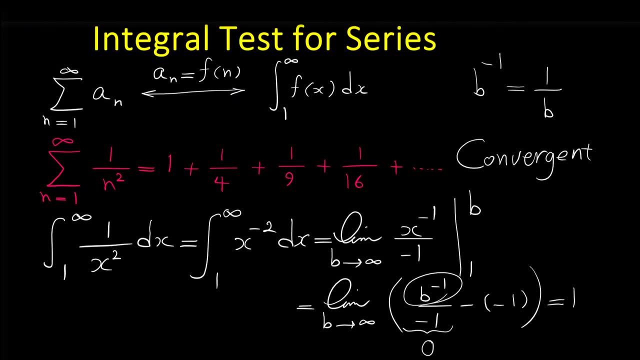 so, as you can see, with this rule immediately, you can figure out the convergence or divergence of these examples. or if you look at the first example that we did here, the power of n is 2 and, based on the p series, when the power is greater than 1. 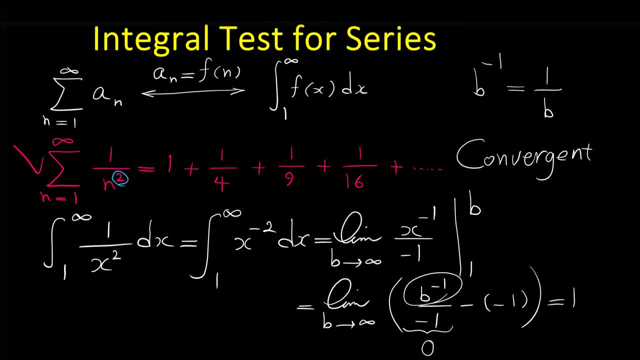 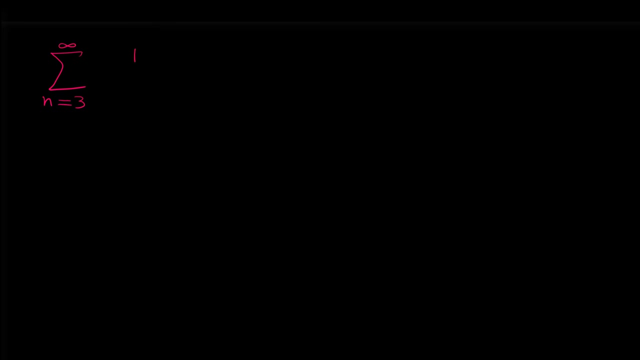 the series is convergent. so i highly recommend you to memorize the rule for p series. p series are convergent for the powers greater than 1 and are divergent for the powers less than equal 1.. let's do another example, sigma n, from 3 to infinity, of 1 over n squared plus 9.. 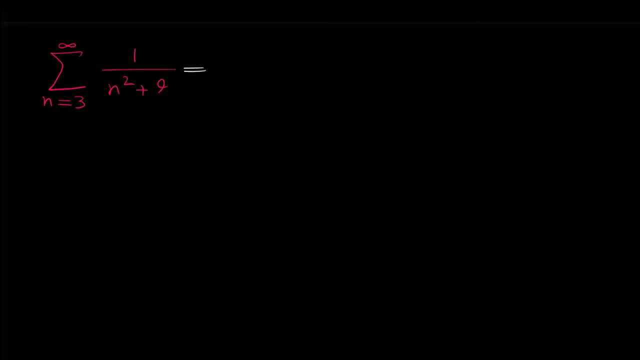 let's do an example of this. if you write the first few terms of this series, it is obvious that the terms of these series are all positive and decreasing. the first term of these series is one over 3 squared is 9 plus 9 is 18- 1 over 18. the second term is 1 over 4 squared is 16 plus 9 is 25- 1 over 25. the third term: if you place on roasting a j is 1 over 18, that's 2, and the third is 6. apply the seventh term and the last is spoilers: 1 over 6. all these j's are positive and all j's are Solar, your. and also 0, because usedados positive corner here in� r1 over 2 is negative. i compared those two, three terms. remember to zoom in and make sure that your at least and all кол-1 is equal fu. Tesla. 1 over 2. very clear, right statement is: the first term is: 1 over 4. squared means 16 plus 9 is 25 way. sai is positive and i'm notcómo. 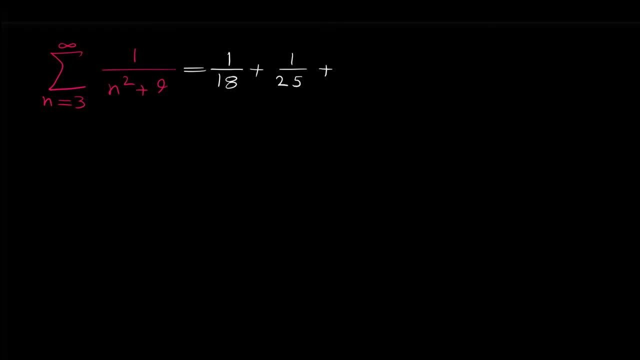 term. if we plug in 5 for n, 5 s squared is 25 plus 9, 1 over 34, and so on. as you can see, all the terms of these series are positive and they are decreasing, so we can use the integral test for this series. the relevant integral to this series is integral from 3 to infinity. 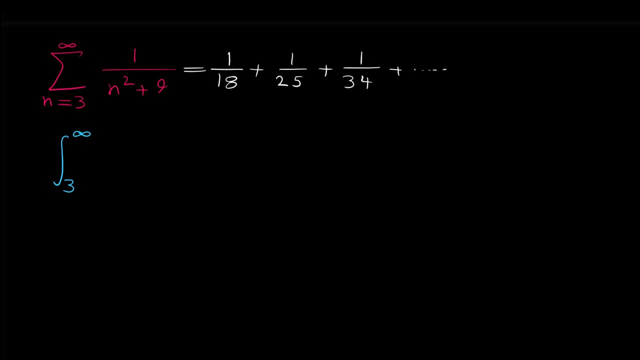 because the series starts from 3, or integral also should start from 3 to infinity- of 1 over x square plus 9 dx. for finding this integral we can use these four formula of the integral integral of dx over x, s squared plus a square which, in this formula, a is: 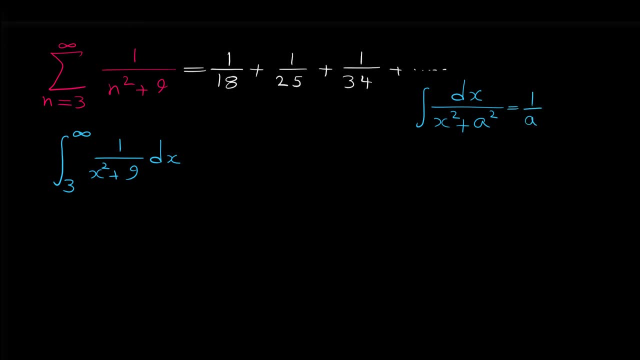 a number is 1 over a tangent inverse of x over a plus c. note that here a s square is 9, and so a is 3, because 9 is 3 s squared and so a is 3, so this integral equals to 1 over 3. 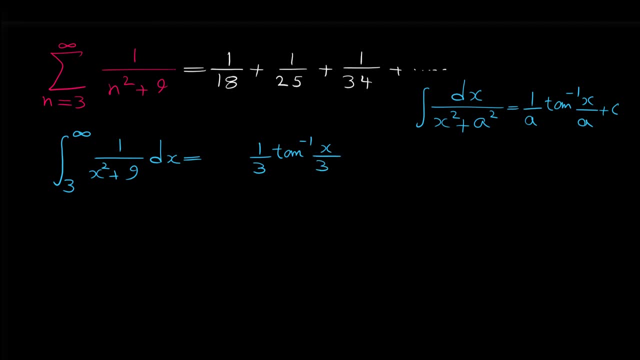 tangent inverse of x over 3. because this integral is improper, we have to write it in the form of three to the b limit, b approaches infinite. if we plug in b, this equals to limit of 1 over 3. tangent inverse of B over 3 minus 1 over 3. tangent inverse of 3 over 2 and B goes to: 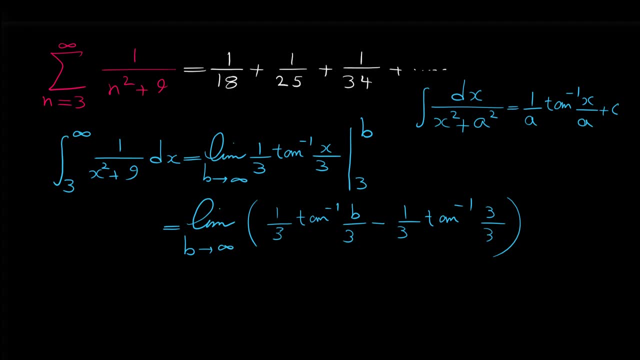 infinity as B approaches infinity, B over 3 approaches infinity and tangent inverse of infinity is pi over 2. we write one-third, and tangent inverse of infinity is pi over 2 minus 1. third tangent inverse of 1, because 3 over 3 is 1, is pi over 4. the angle whose tangent is 1 is pi. 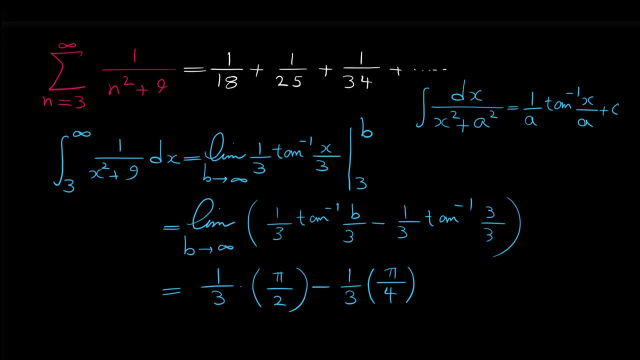 over 4, I over 2 times 1 third is pi over 6, and pi over 4 times 1 third is pi over 12. if you do a simple calculation here, this equals pi over 2, because the integral is convergent based on. 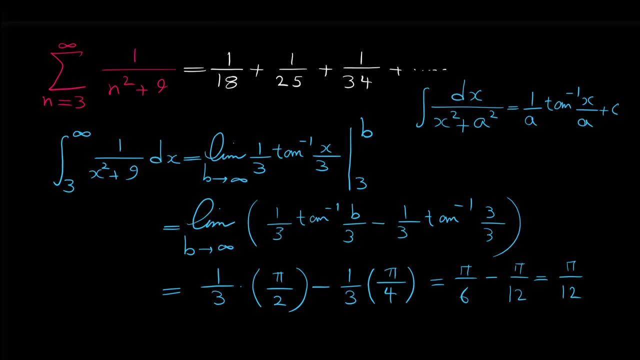 integral test. the series is also convergent, so this given series is a convergent series. but note that we don't know to what value this series converges, and only we know that it is convergent.